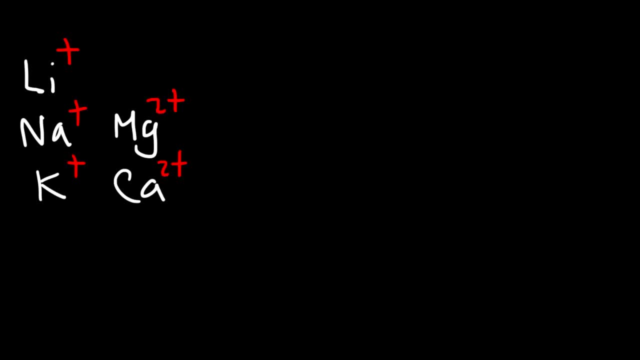 plus charge. Now, in the middle you have transition elements which can have variable charges, So we're not going to focus on those too much. but moving on to group 13, also known as group 3a, you have elements such as aluminum. I'm going to write it over. 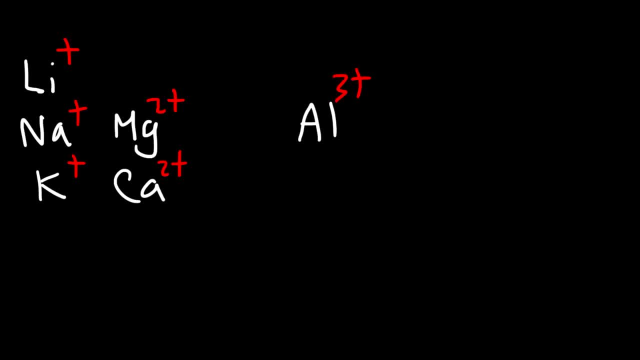 here, and this element has a 3 plus charge. and then you have elements like carbon, silicon, germanium, which are found in group 4a and for ionic compounds. it's rare that you'll see those elements In group 5a. you 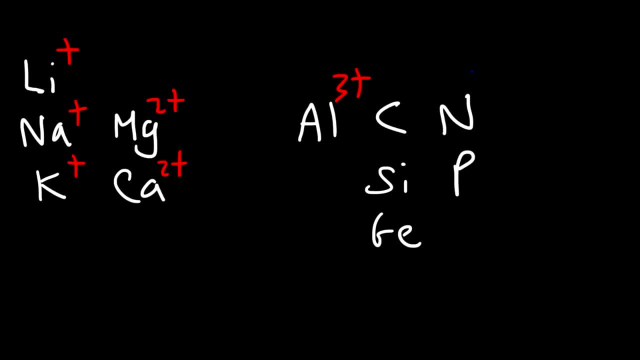 have nitrogen and phosphorus. These form negative charges, specifically minus 3 charges. and then you have elements like oxygen, sulfur, selenium. These are the calcogens which form a negative 2 charge. and finally you have the halogens like fluoride, chloride, bromide and iodide, And these halogens, they form 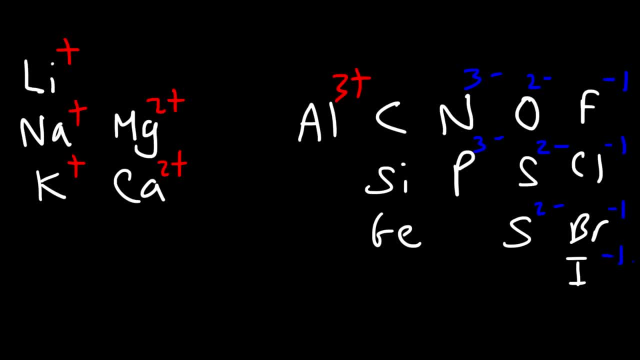 anions with negative 1 charges, And so make sure you understand how to determine the charges of ions for certain elements using the periodic table, because that's going to be important. Now let's start with our first example. Let's say, if we want to write the 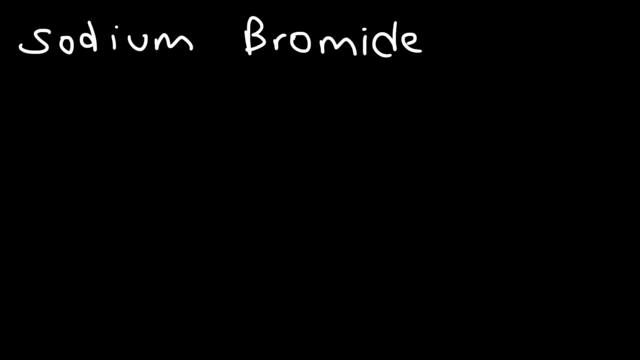 chemical formula that corresponds to sodium bromide. How can we do so? The first thing we need to do is list the ions that are involved here. The sodium ion has a positive 1 charge and the bromide ion- it's a halogen- it has a negative 1 charge. So how can we use this? 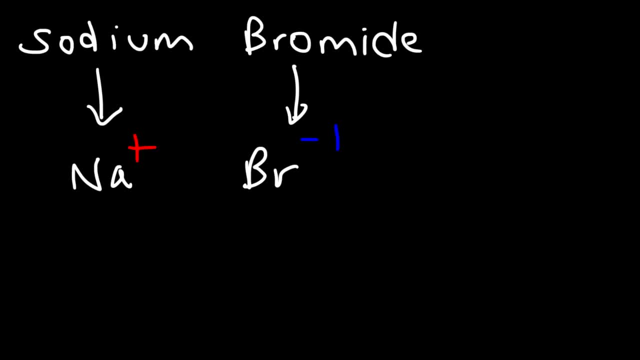 information to write the chemical formula of sodium bromide. Now, if the charges are the same in magnitude, even though they're opposite in sign. so like this is plus 1, this is minus 1, if the charges are the same, these ions will combine in a one-to-one ratio, so you can simply write: 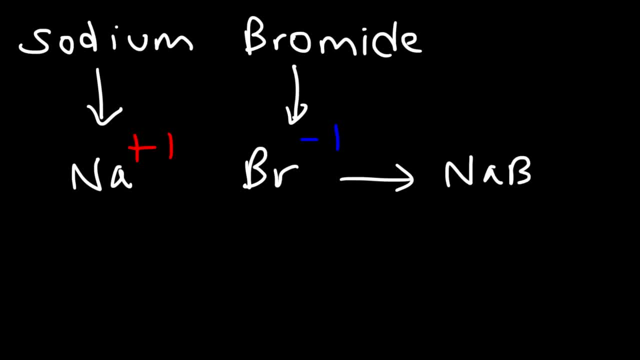 them together as NaBr. So that's the answer for this example. So anytime the magnitude of the charges are the same, you could just write the elements together. Let me give you another example of that. So let's say, if we want to write the chemical formula for calcium sulfide Now, 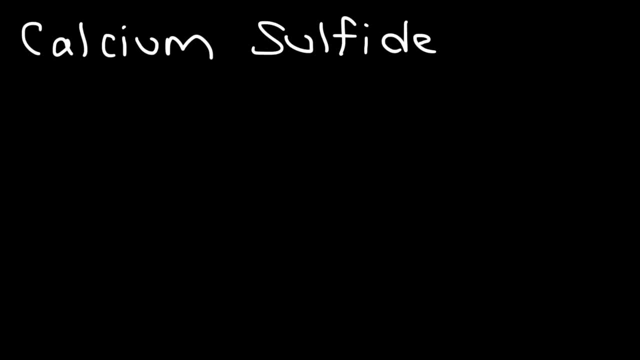 the first thing we're going to do is write the ions. So calcium is an element in group 2, so therefore, as an ion, it's going to have a 2 plus charge. Sulfide is a chalcogen in group 6a, so it's going to have a 2 minus charge. 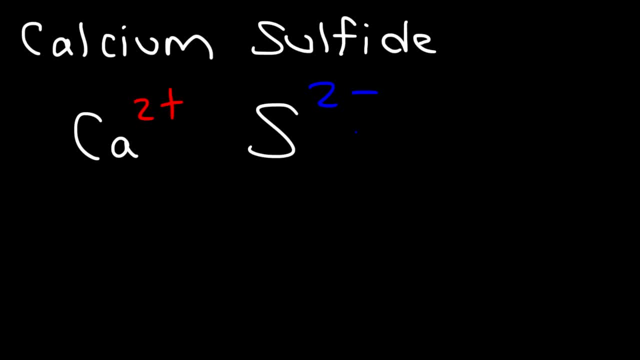 Now notice that the magnitude of the charges are the same- 2 plus and 2 minus- So you can simply write them in a one-to-one ratio. This is going to be CaS- calcium sulfide. That's the answer for this example. Now let's try another similar problem: Aluminum phosphide. 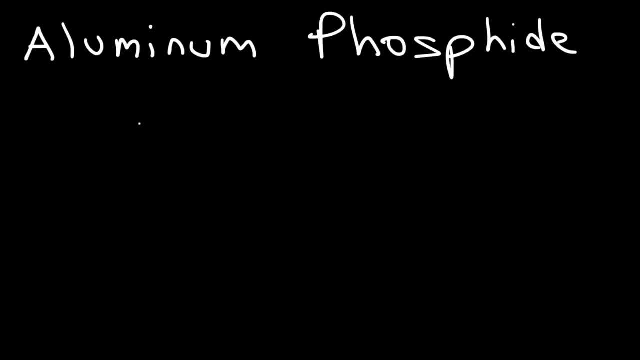 So what is the charge on the aluminum cation? Aluminum is found in group 13 or group 3a, So it has a 3 plus charge And the element phosphorus has a negative 3 charge as an anion. So writing them together, the answer is simply going to be Alp, because they have the same. 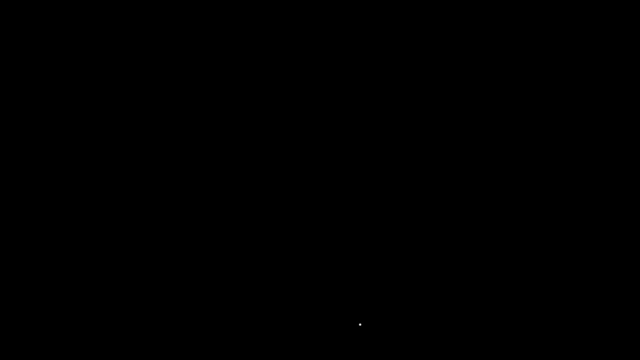 charge magnitude. But now, what if the magnitude of the charges? what if they're different? What if they're not the same? So what do we do in a situation like that? So, for instance, let's say, if we want to name aluminum chloride, Let's try this example, So we know that aluminum has a 3 plus. 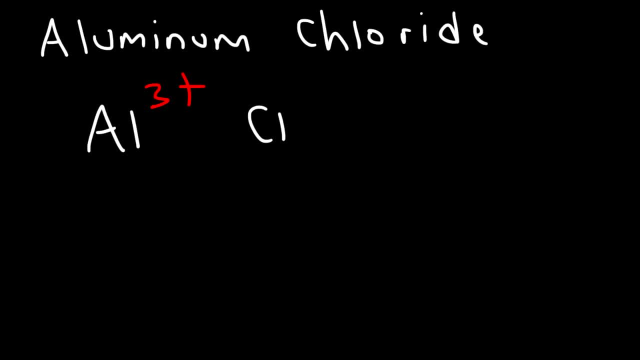 charge and chloride is a halogen with a negative 1 charge. So how do we work with this? Now, there's a technique that we could use. We need to swap the charges with the subscripts. So let me show you. So this 3, we're going to write it as a subscript towards the right. 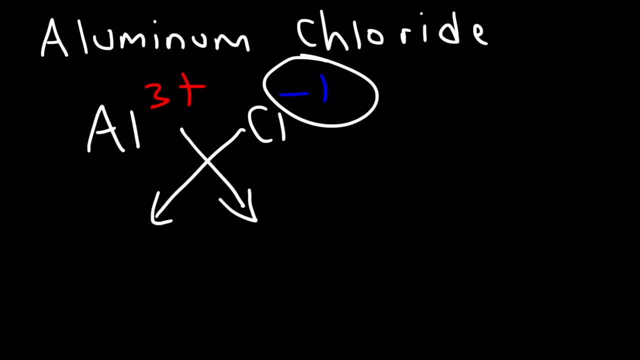 And the 1, not including the negative sign. we're going to write it as a subscript to the left, So this is going to be Al1Cl3.. Now there's no point in writing a subscript of a 1.. So in this case we can just omit the 1 and say AlCl3.. It turns out that this is the correct. 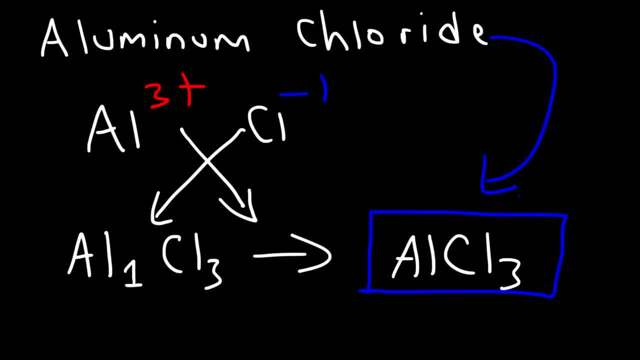 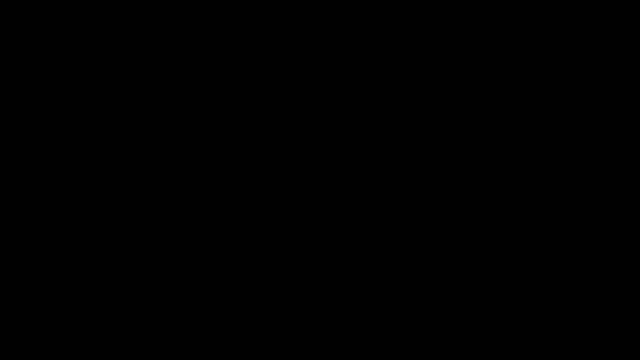 chemical formula for aluminum chloride. Now let's make sense of it. So why do we need the 3?? The answer is to balance the charges. We have one aluminum ion with a 3 plus charge, So the total positive charge in this compound is positive 3. To balance that 3 plus charge. 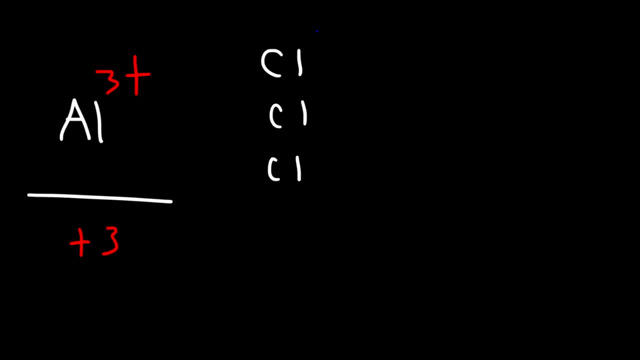 we need three chloride ions, each with a positive charge. So we're going to use Al2Cl3. And we're going to add a negative 1 charge, So that the total of all the negative charges is minus 3.. So these cancel and they add up to 0. And so that's why the chemical formula is AlCl3.. 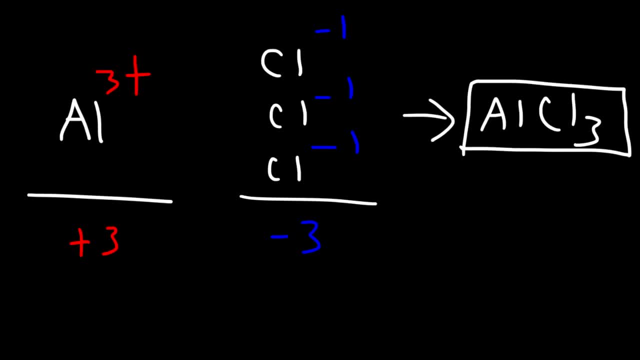 It's to neutralize the charges. We need three chloride ions to neutralize the one, aluminum plus 3 cation. Now let's work on some more examples. The next one we're going to use is Al2Cl3.. The next one we're going to try is sodium oxide. 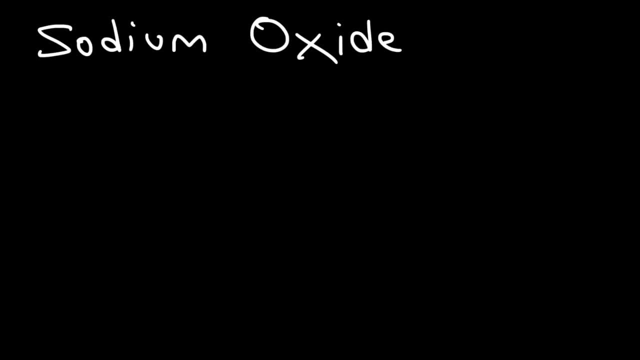 What is the chemical formula that corresponds to this compound? So let's start with sodium. It's Na+. Now what about oxide? So we have the element oxygen, and oxygen is a chalcogen in group 6A, so it's going to have a negative 2 charge. 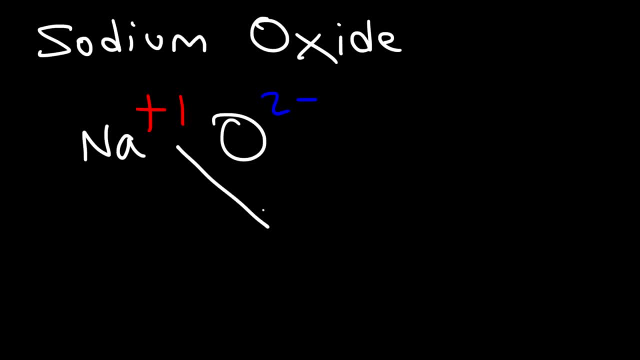 So, using the method that we used before, we're going to swap the charges with subscripts, So it's going to be Na2O1, or simply Na2O. So this is the answer. So this means that we need two sodium cations to neutralize the oxide ion. 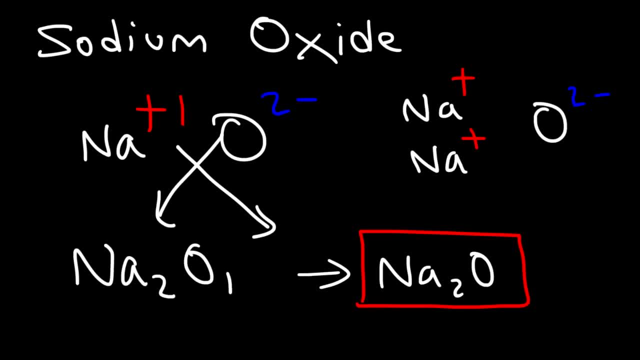 The total of all the positive charges will be plus 2, and the total of all the negative charges is minus 2.. So that's why we need two sodium cations to balance the negative 2 charge on the oxygen, And so this is the answer: Na2O. 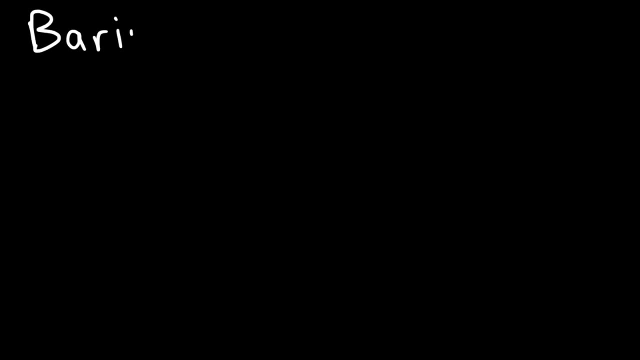 Now let's work on this example: Barium phosphate. Feel free to pause the video if you want to, If you want to work on that problem Now. barium is an alkaline earth metal found in group 2, so it's going to be Ba2+. 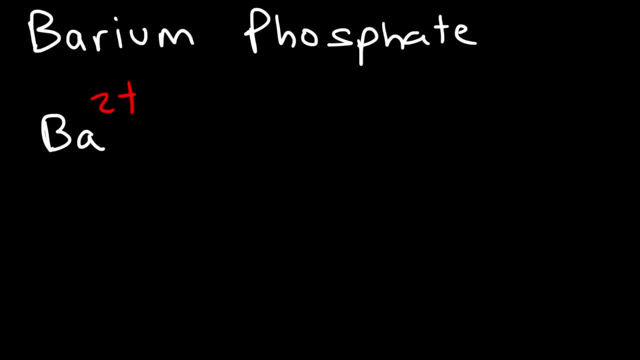 And phosphate is a polyatomic ion which is PO4 3- And the polyatomic ions. you need to commit that to memory Now I've created a video on YouTube and you can search it out. Just type in polyatomic ions- organic chemistry tutor in the YouTube search bar. 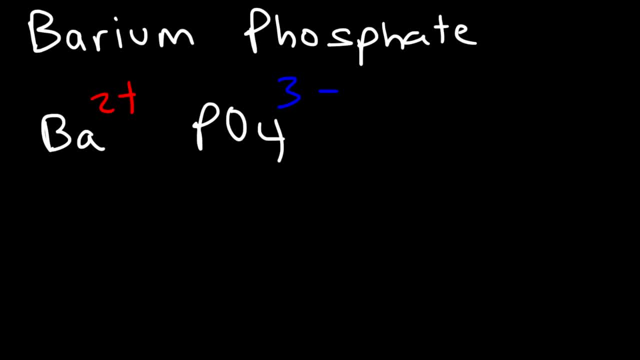 And you can get a list of polyatomic ions that you need to know. So make sure to take a look at that. Now, using what some call the crisscross method, this is going to be Ba3PO4 times 2. But because we have a polyatomic ion, because we have multiple polyatomic ions, rather, 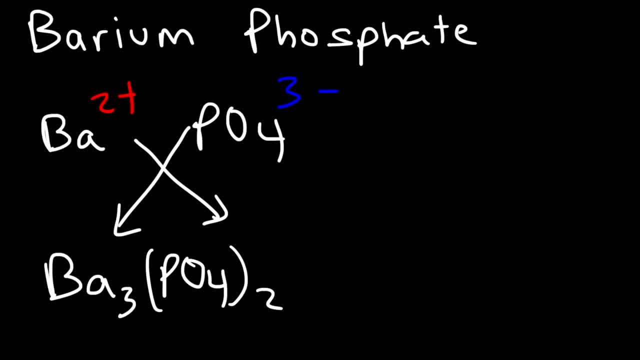 we need to enclose the PO4 ion in parentheses, And so that's how you can write The chemical formula for barium phosphate. So anytime you have multiple polyatomic ions, make sure you surround it in parentheses. Now the last case will be one with a transition metal. 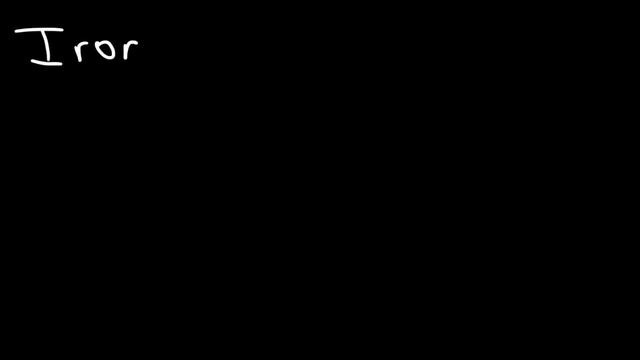 So let's say, if we have Iron 3, sulfate, How can we write the chemical formula for this compound? Now it's important to understand that the Roman numerals that you see here tells us the charge on the metal. so iron has a 3 plus charge and sulfate is. 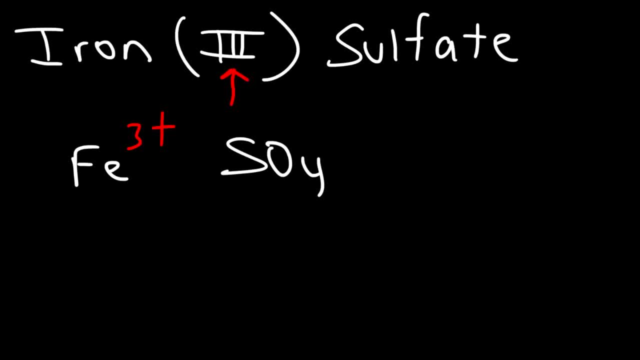 a polyatomic ion which, you need to know, is SO4 2-. so with this information we can swap the charges with the subscripts. so it's going to be Fe2SO4 3 and that's basically it. so now you know how to write the chemical formula of ionic.